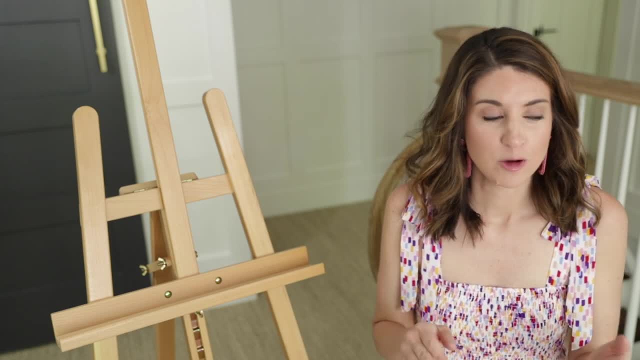 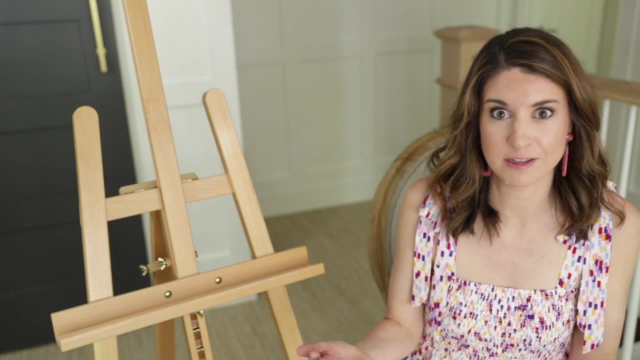 neutral colors are so hard to get right. So with grayish you're either dealing with green, which is the majority of the grayish paint colors on the market, and a lot of people freak out when I say that gray has a green undertone. but don't worry, That is the most neutral undertone of all the gray. 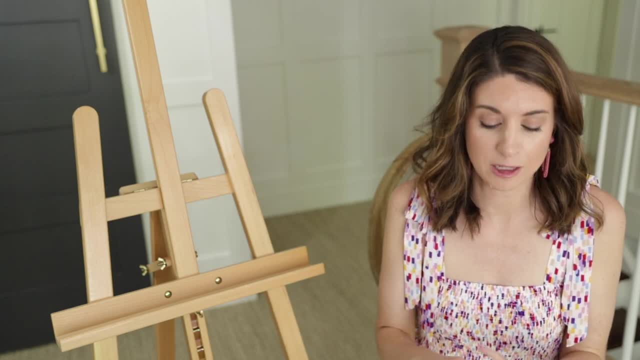 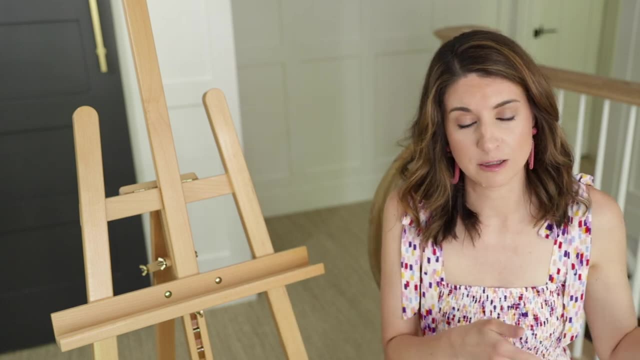 undertones to deal with. So you've either got gray, you've got violet or you've got blue. There are no grayish with blue undertones. That's just too cool. Those are considered blue grays. Don't let anyone tell you that repose gray is a grayish, because it's not. It's a blue gray. 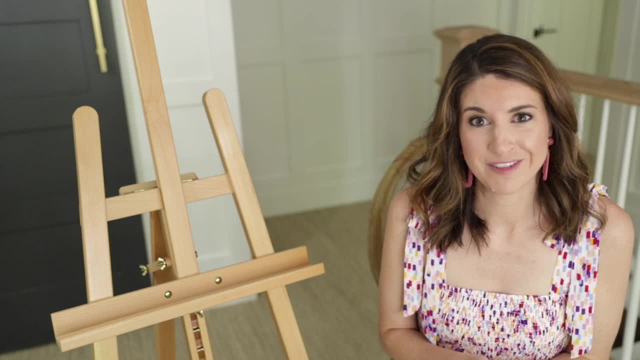 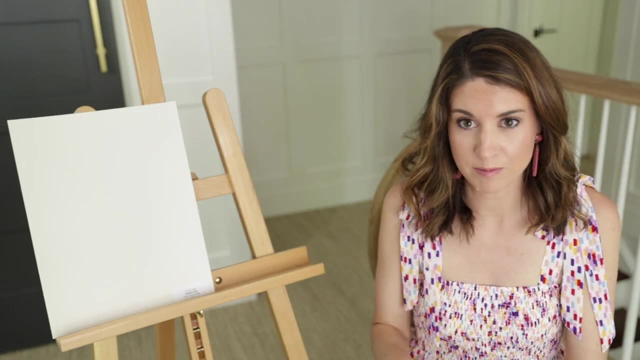 So now that you know undertones, let's get into my favorite grayish colors. Benjamin Moore Classic Gray. This is the lightest paint color on this list. If you're familiar with light reflectance value, it has to do with how light or dark a paint color. 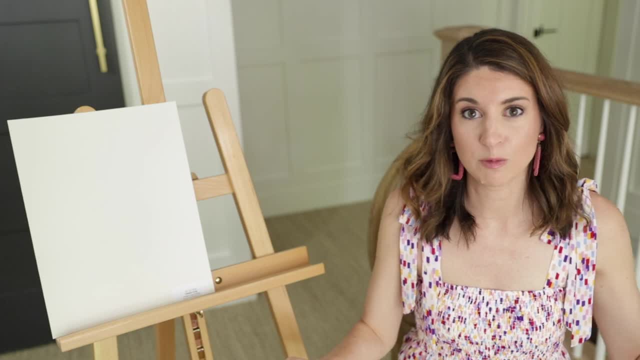 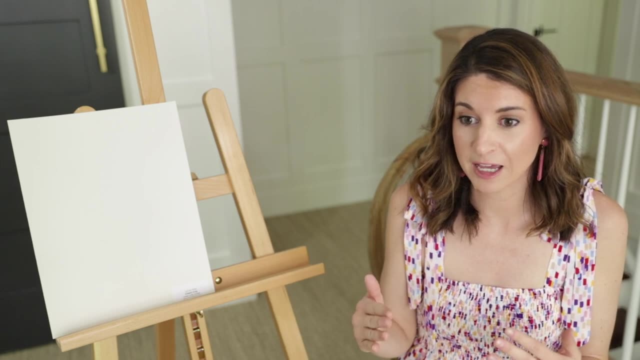 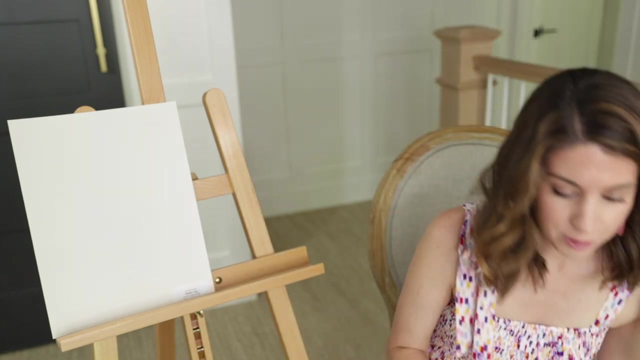 is, with 100 being absolute pure white and zero being absolute pure black. This is, this sits at 75, so it's pretty light. It's not as light as off-white, which a lot of people think- that classic gray is an off-white. I actually have an off-white. Let me show you that. 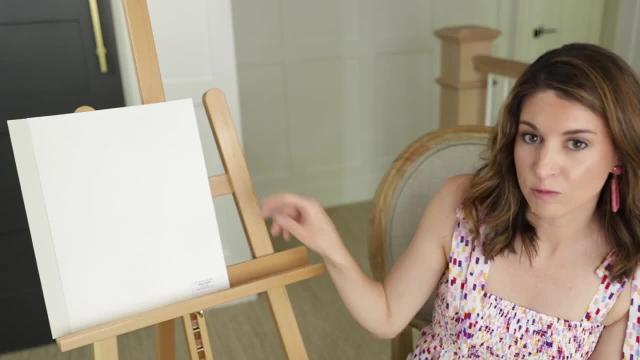 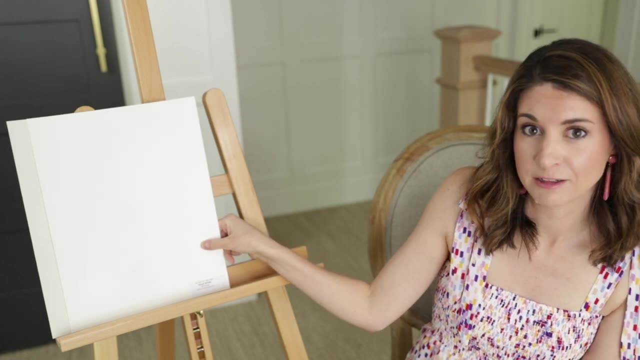 Okay. so when you compare it with cloud white, which is a true off-white- and I think it's LRV sits around 84-ish- you can easily see that this is not that. classic gray is not an off-white. It is a grayish paint color with a green undertone. 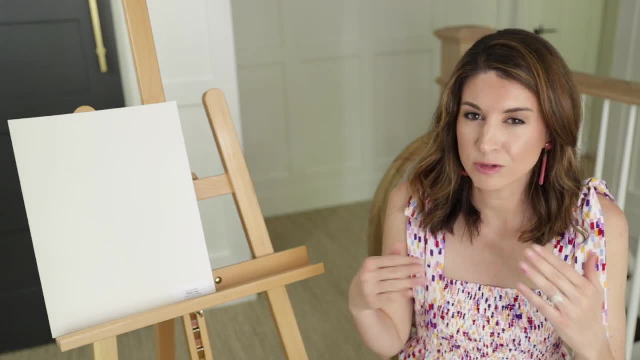 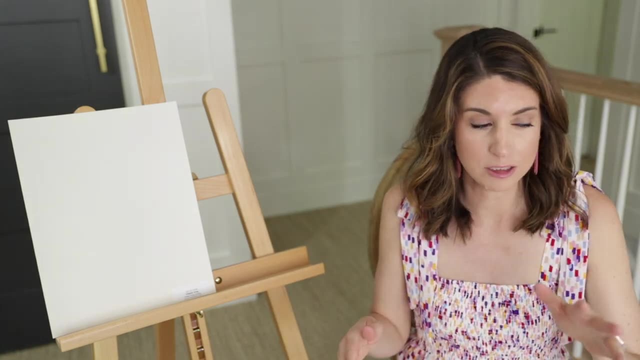 fairly neutral, but it doesn't work with everything. It doesn't really look very good with earthy kind of finishes. So if your home was built in the 80s, 90s and you have, or early 2000s and you have kind of like that Tuscan trend going on, you've got the terracotta tile. 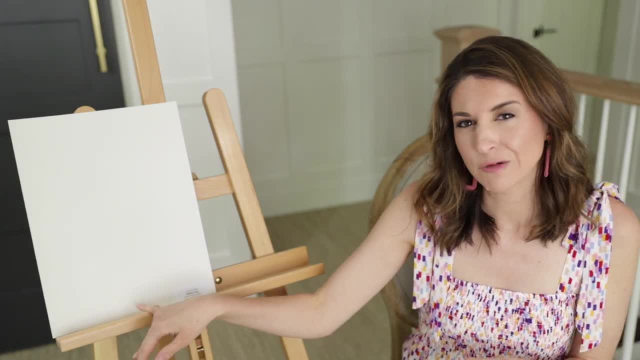 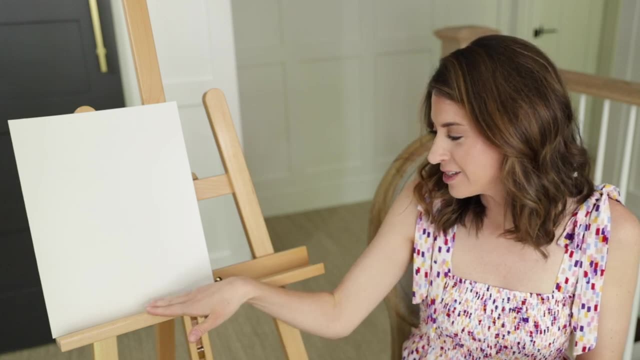 you've got the brown granite. this is not really going to be the color to update your home. You're going to want to look more at like taupe grayish, which we'll cover later on. So this is Benjamin Moore Classic Gray. 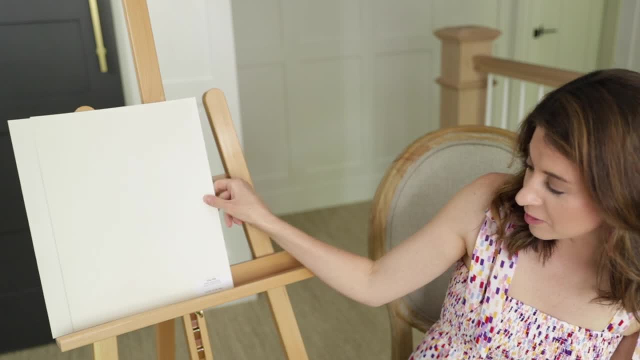 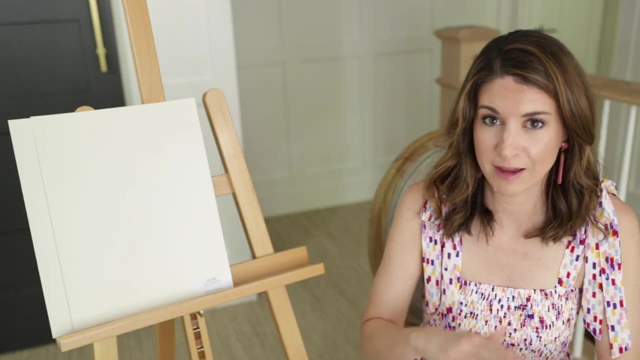 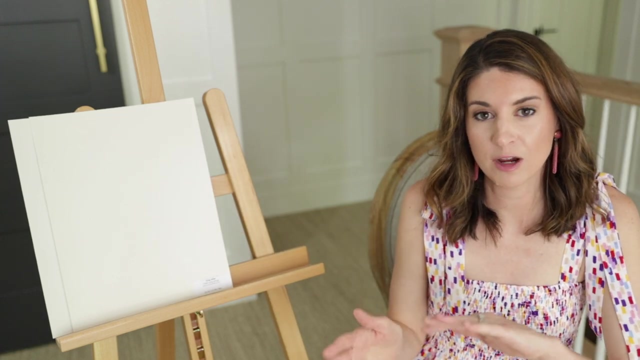 Benjamin Moore Gray Mist- Another grayish with a green undertone. It's just, it's LRV is 74 when compared to 75, so not too much of a light depth difference there. It's got a little bit more beige. So some of the grayish you'll find lean a little bit more to the gray side and some lean a. 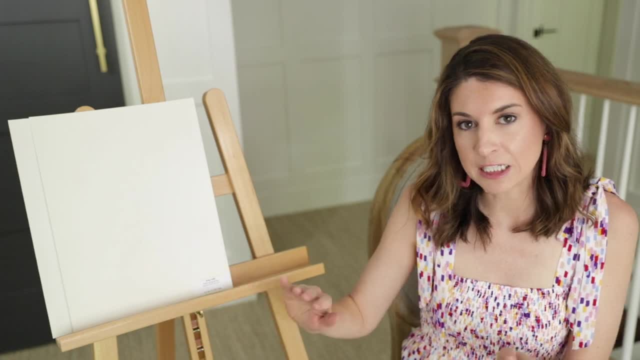 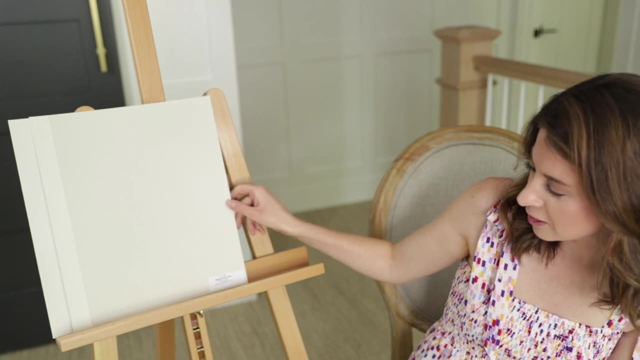 little bit more to the beige side. Gray Mist, to me, is one that leans a little bit more to the beige side. Benjamin Moore, Edgecomb Gray. I'm sure you've heard of this Super popular paint color. It's still considered a light paint color but comparatively speaking to 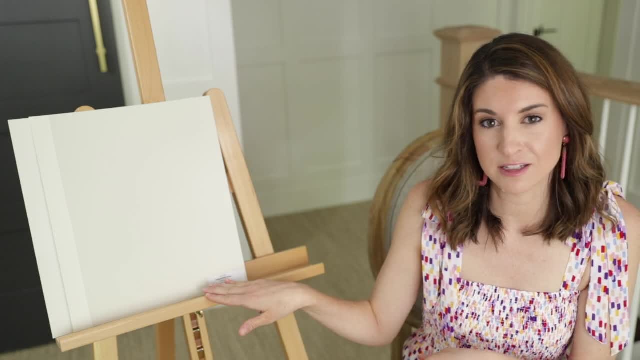 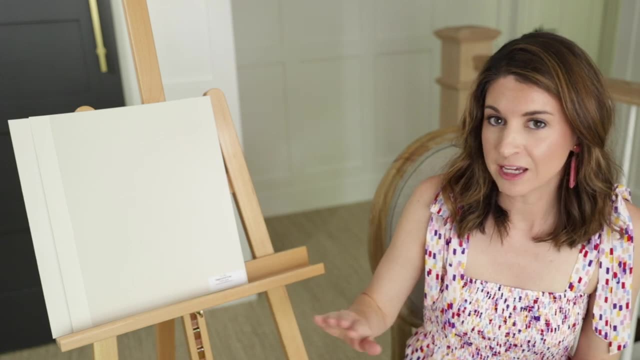 the first two that I've shown you. it's LRV sits at 63, so it's much darker. It's still pretty light and airy. It does have a green undertone. It kind of again like which one did I do Gray Mist It. 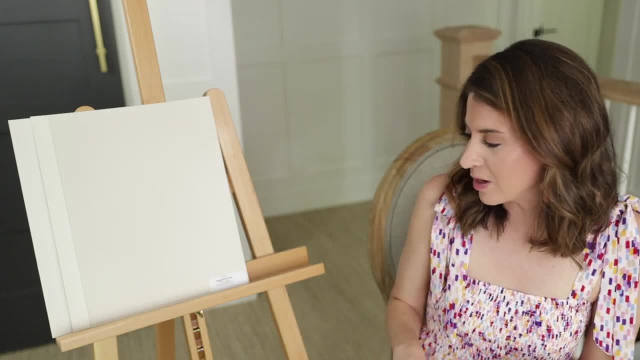 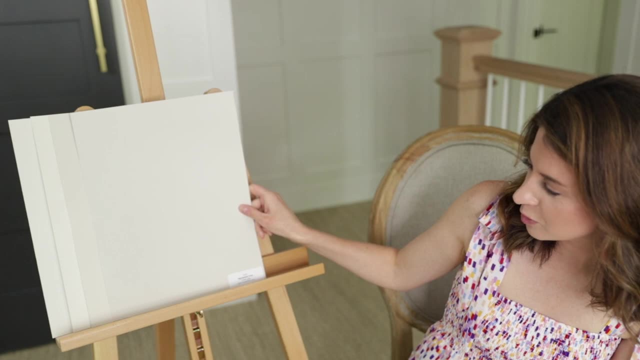 leans a little bit more to the beige family, but it's really really pretty, really soft on walls. Sherwin-Williams Agreeable Gray- Another pretty popular paint color. It's got that green undertone. It's not quite as pronounced as. 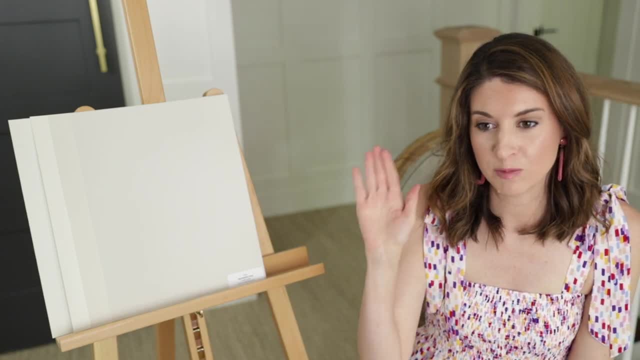 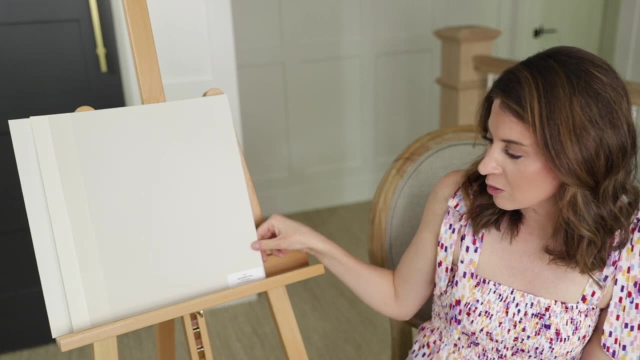 Edgecomb Gray. You'll see that gray come out. if you paint this on your wall and you've got a lot of purples and blues, immediately that green will come out. It's a little bit darker than Edgecomb Gray, but not too too much, So that's Agreeable Gray. 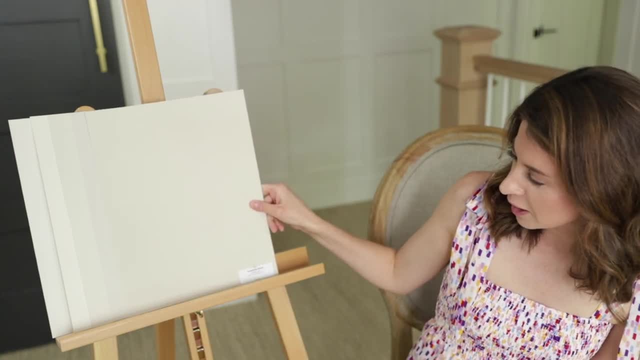 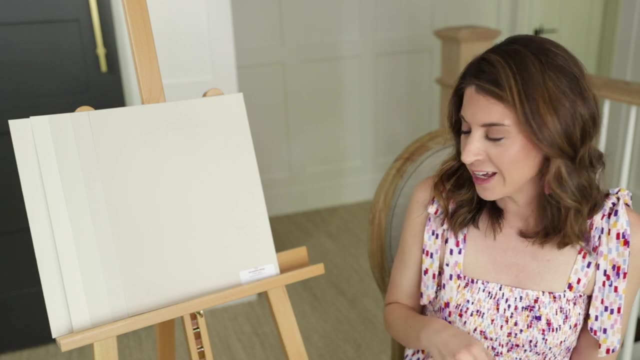 Sherwin-Williams Accessible Beige. Oh, this color was all the rage several years ago. We have it downstairs. We'll be repainting because we got new furniture and it totally clashes. but this is Accessible Beige. It's a little bit darker, a little bit more saturated than some of the other colors on the list, especially. 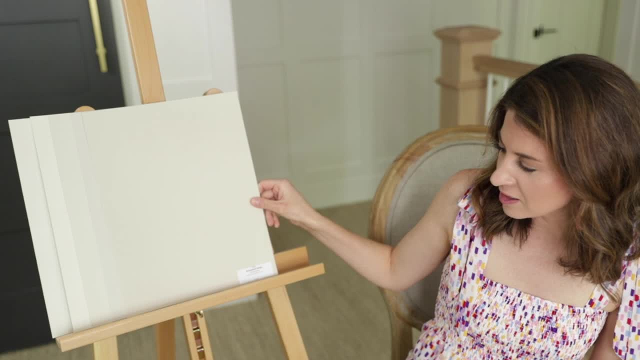 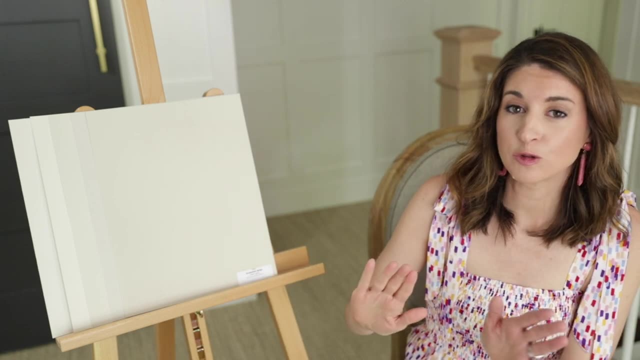 when you compare it to Classic Gray and Gray Mist, I think the LRV sits at 58. It's got that green undertone, like a lot of these grayish colors, And, as you can see, it definitely leans more towards the beige side of. 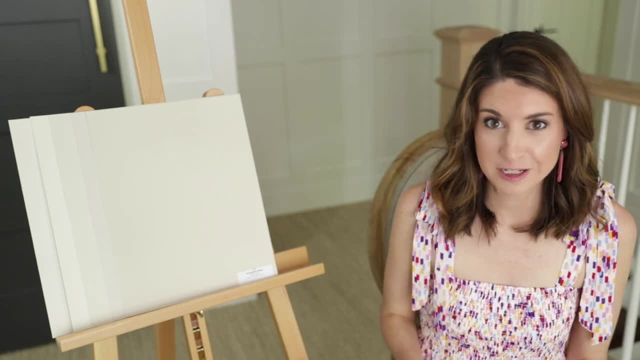 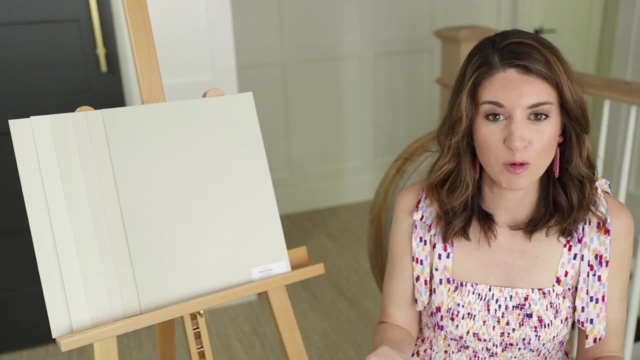 things. So that's Accessible, Beige. Okay. so I couldn't do this list without Benjamin Moore, Reverre Pewter. So for a while, you know, you would ask people what paint color they were thinking. you know what color. 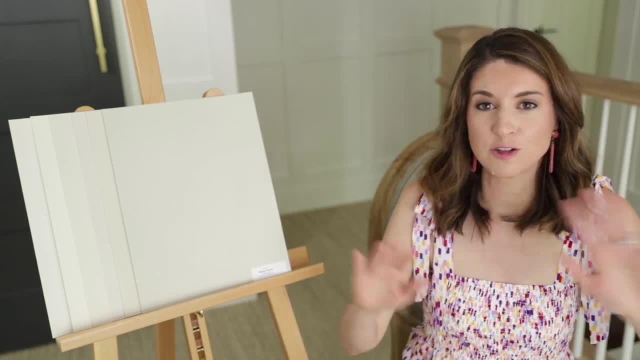 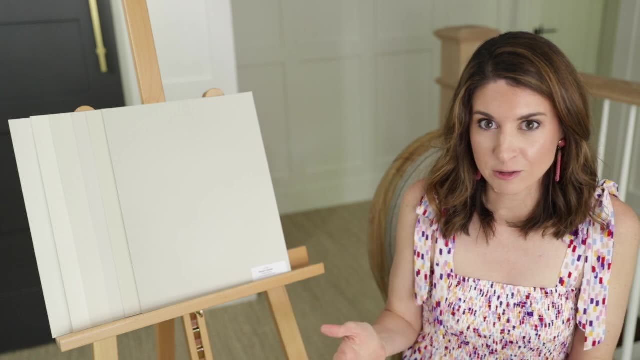 they wanted. Everyone was just Reverre Pewter. It was like the answer to everyone's design dilemma. So it's a pretty neutral grayish color. It's got that green undertone which makes it pretty easy to work with. Now it doesn't work in all situations or all homes, but it is fairly easy to work with. 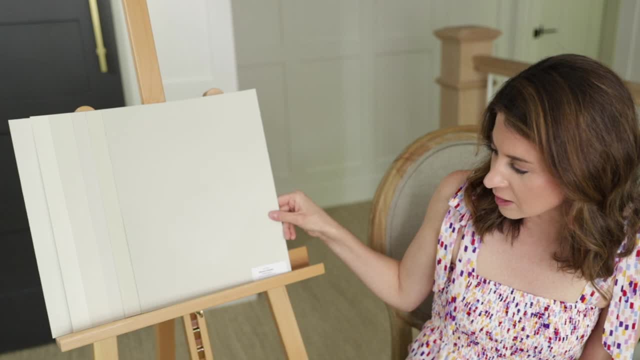 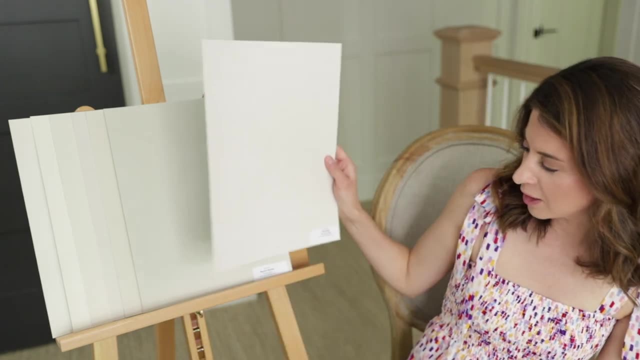 It's more saturated. It's probably the darkest color on this list just by a little bit. But that is Benjamin Moore- Reverre Pewter. Benjamin Moore- Pale Oak. So now we're getting into a little bit of a different undertone family. 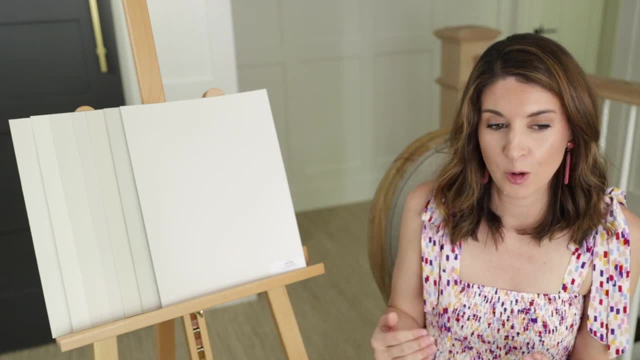 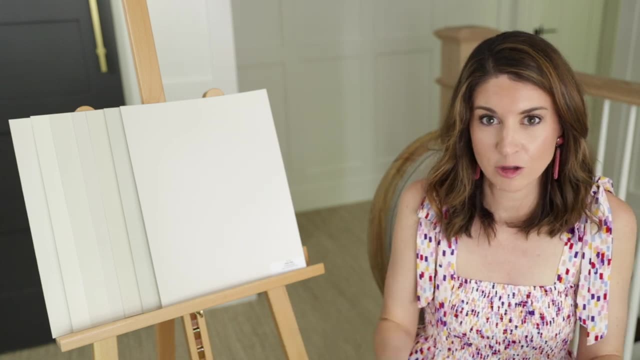 So this is technically a taupe grayish. So a lot of people like those taupe colors because they're warmer than the grays but they're cooler than the beiges. So it's kind of like that good in-between warm color. 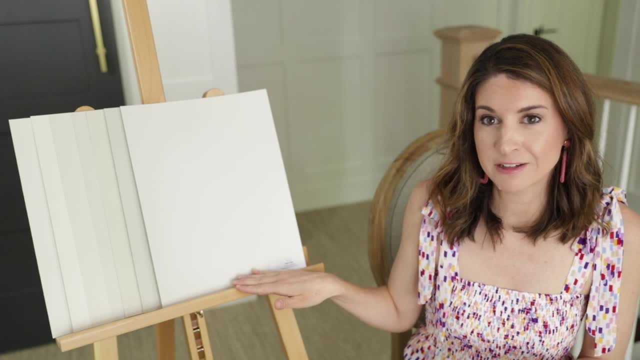 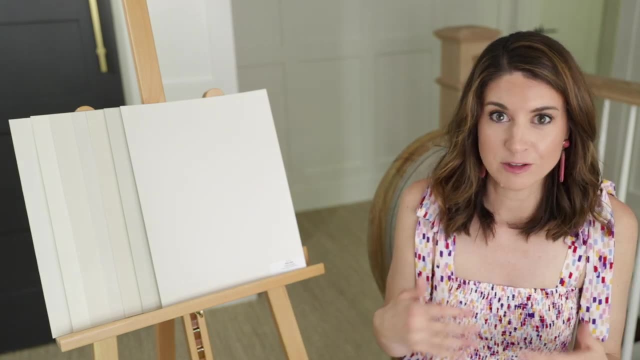 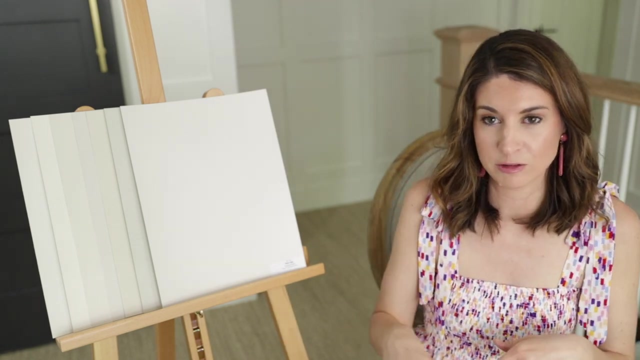 But they're not for every spaces because taupes can be a little bit tricky to work with. They've got that pinky purple undertone And that's again why it's not for every space or every room, But just so you know, taupes the undertone always leans pinky purple, or either pink or purple. 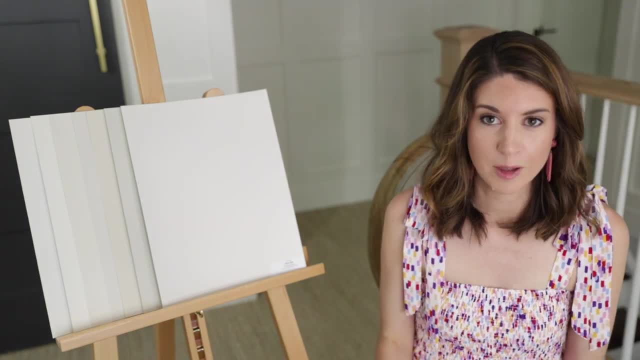 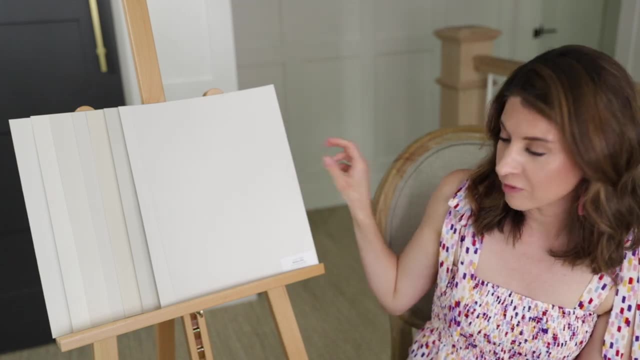 So that's something to be aware of when you're looking at taupe grayses. Benjamin Moore Balboa Mist. This is a pretty light paint color. Its LRV sits at 67, so it's not quite as light as some of the early ones that I showed you. 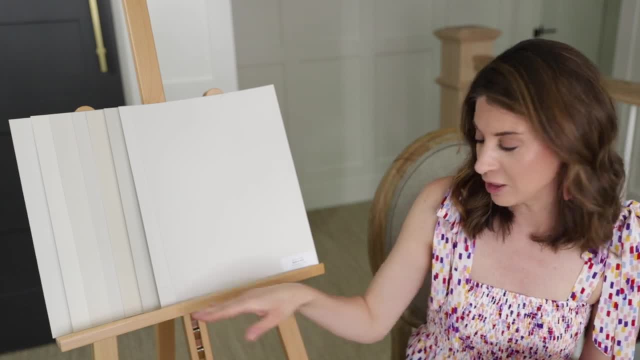 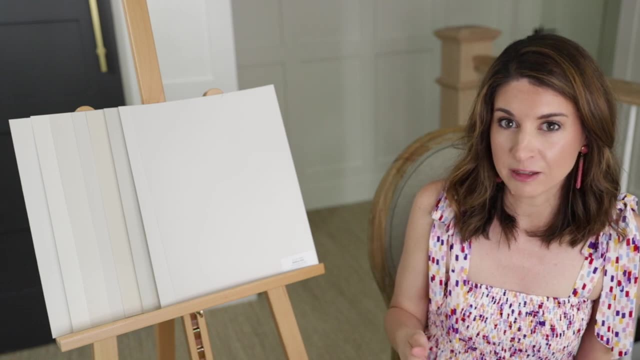 but it's definitely not as dark as Edgecombe Gray and Accessible Beige. Balboa Mist is actually a grayish with a violet undertone, So a lot of people think that they need something like Balboa Mist, when actually they need more of a taupe. 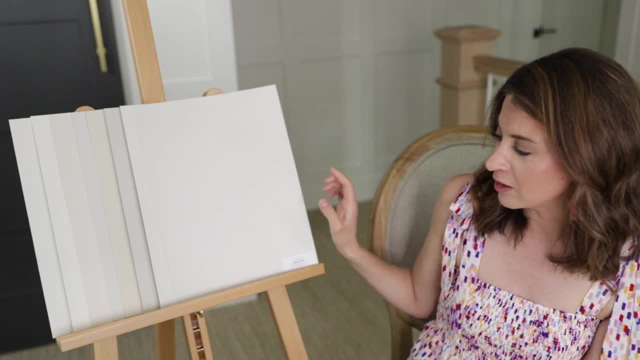 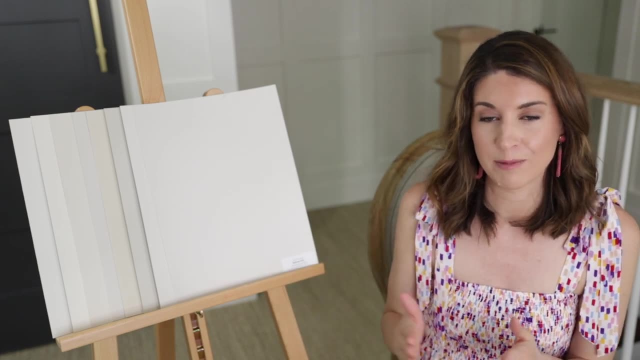 So that's just something to be aware of when you are looking at these neutrals. That's why it's so important to compare, compare, compare multiple colors, And there's a lot of fabrics that have violet undertones. You would be surprised. 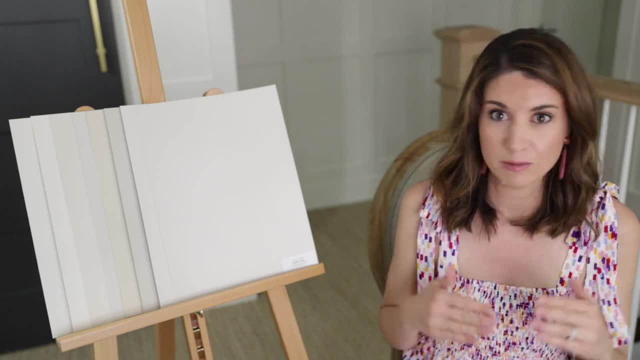 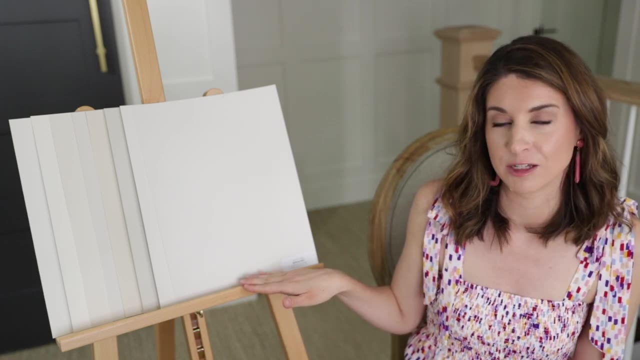 When I tell people that you need a gray with a violet undertone, they look at me like I'm crazy. But in reality a whole lot of fabrics have those violet undertones Which work really, really nicely with those violet, gray, grayish paint colors. 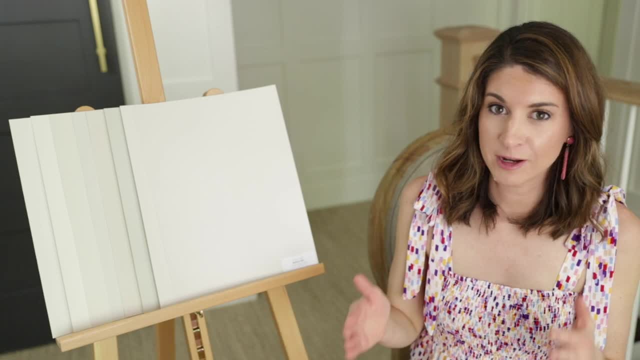 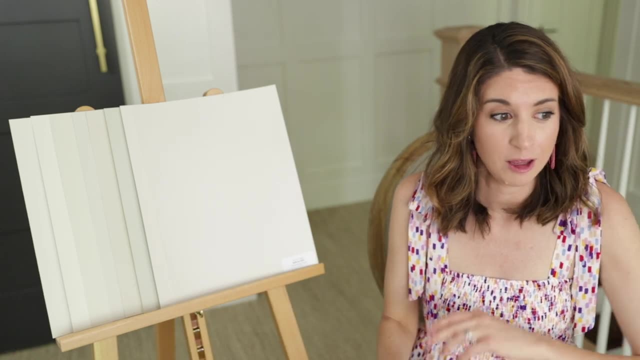 Okay, so now we're going to talk about the hard part: Figuring out which grayish is right for your space And is grayish, even the color you need. You might need a beige, You might need just a taupe, You might need a gray blue. 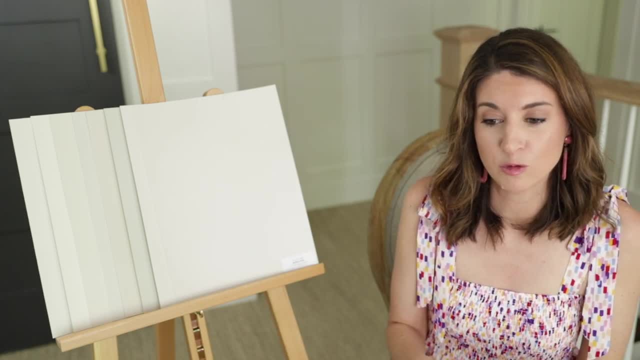 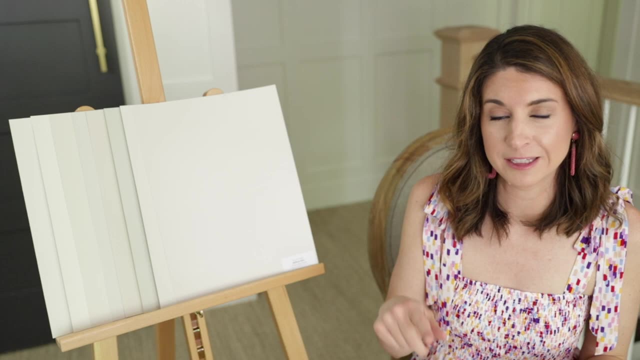 So we're going to try and break that down real quick. If you really want to get into the weeds of this, I have a perfect blog post on how to determine the right paint color for you. I'll link that below And that will really kind of help you kind of solidify some of these concepts. 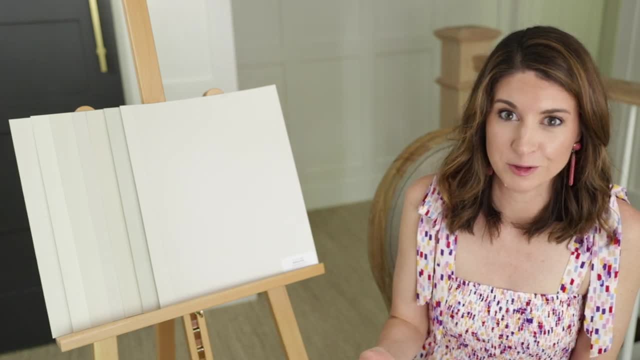 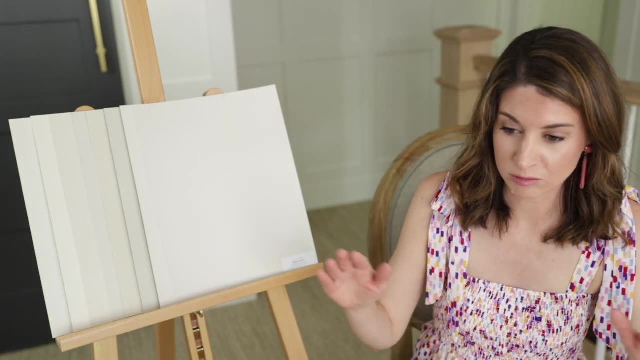 Because I know it's really it's really difficult to understand if this is your first time hearing it, So let's get into it. So, what you want to do, the first thing you want to do when you are comparing, when you are looking for a neutral paint color, 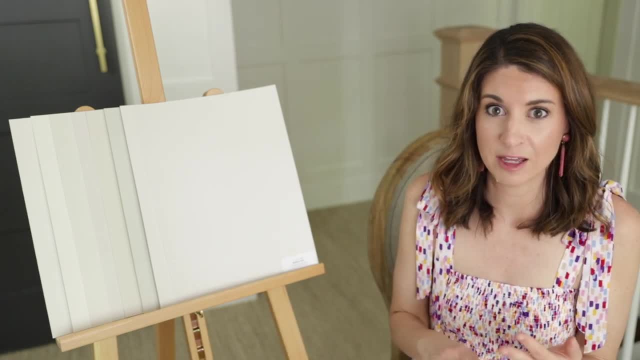 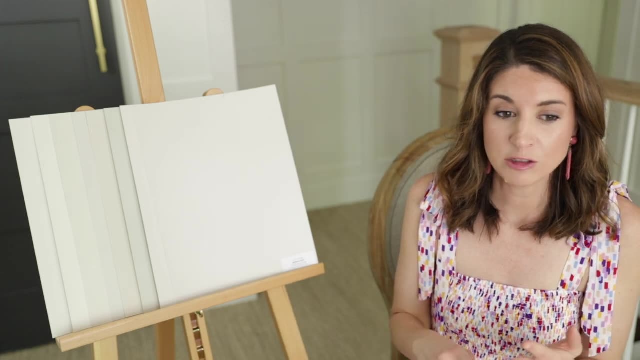 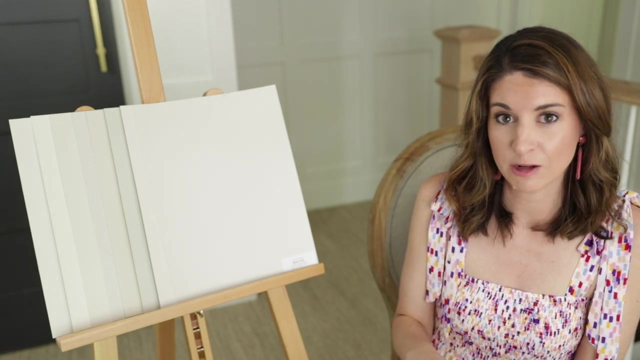 Is to first go around your room and identify the fixed elements and the furnishings, Basically anything that would be too expensive to change. You need to go around and you need to see what the undertone is. So with your couch, if it's a neutral kind of couch, you need to evaluate it for the undertone. 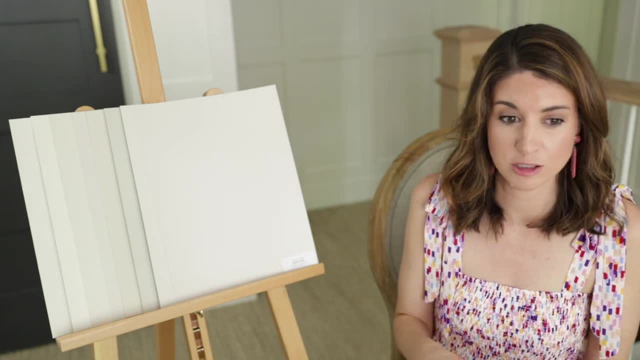 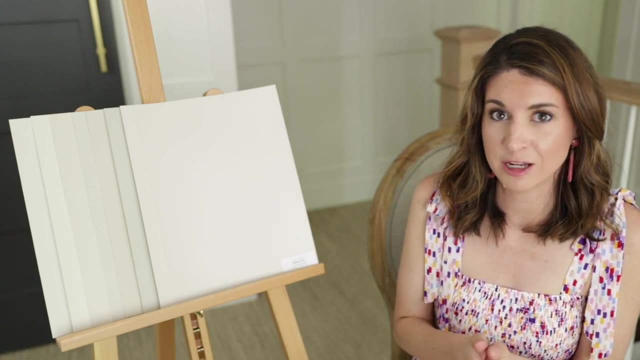 You need to look at your countertop, Look at your cabinets, Look at your backsplash. Anything that again cannot be changed. you need to evaluate it for the undertone And then you need to start sampling colors and comparing to see how they react to that undertone. 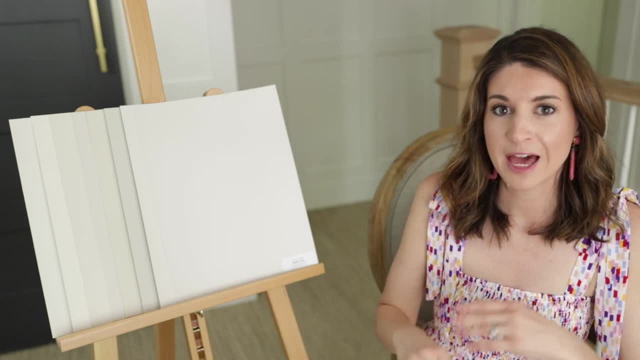 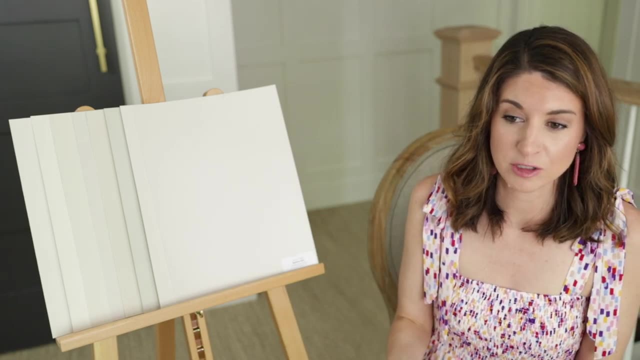 So do they match it? Do they clash? That is really the best way to determine the neutral paint color for you, Don't? you know grayish can be bad. You know grayish can be misleading, because a lot of people just think that they are the answer. 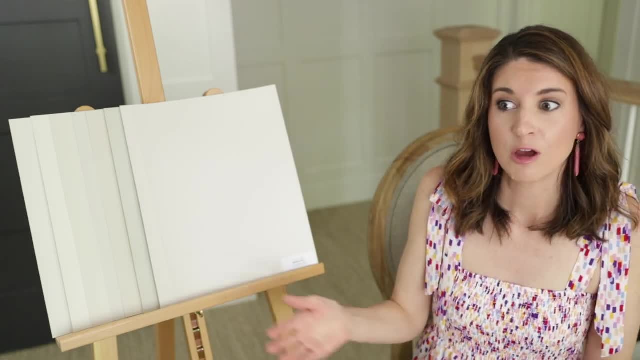 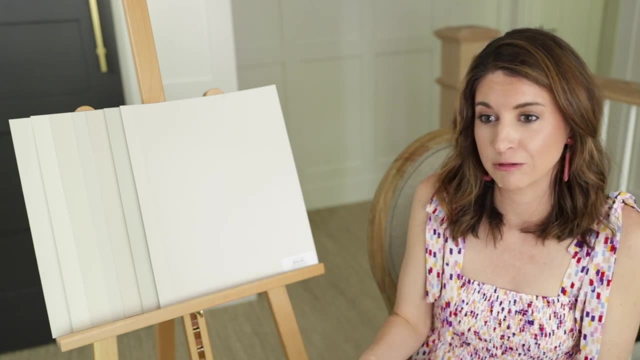 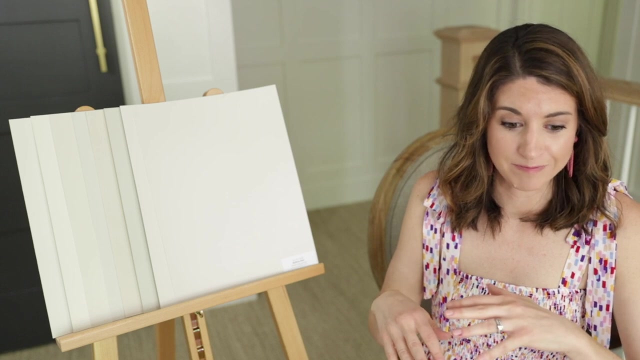 Like I just want something warmer. So any grayish will do, When in fact they really have more of a beige kitchen and they really need more of a beige, maybe with a green undertone wall color. So that's why you really can't go off of color names or kind of ideas about color families. 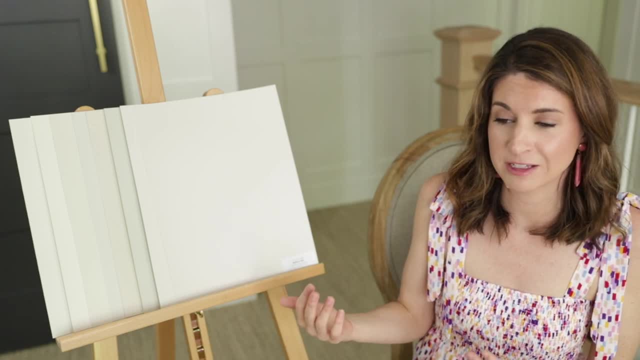 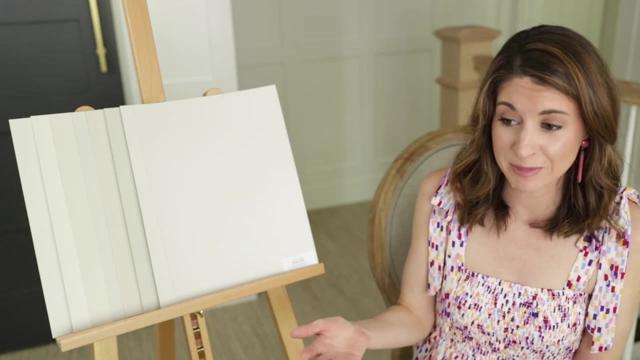 You really have to test these colors out and compare them to your fixed elements So you might realize that you have several different undertones in your room, and that happens a lot, So you'll just need to look at the undertones of whatever is most dominant. 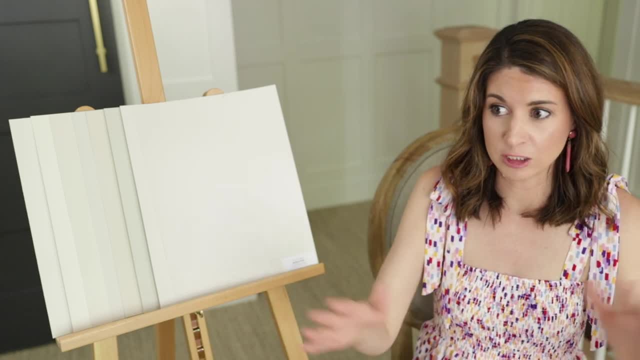 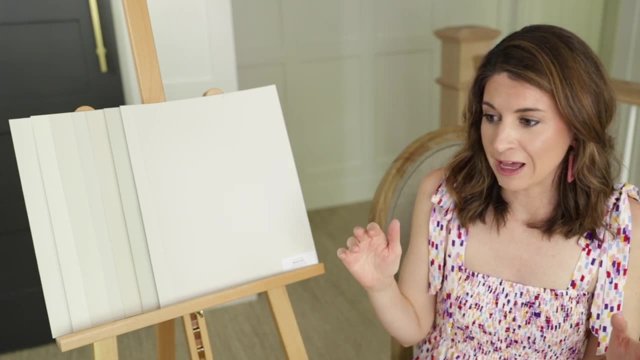 So if you have a fireplace in your living room and you're looking for a, say, you have a stone fireplace and you're looking for a whole room color, But then you also have a small couch that you could potentially- you know- get rid of, 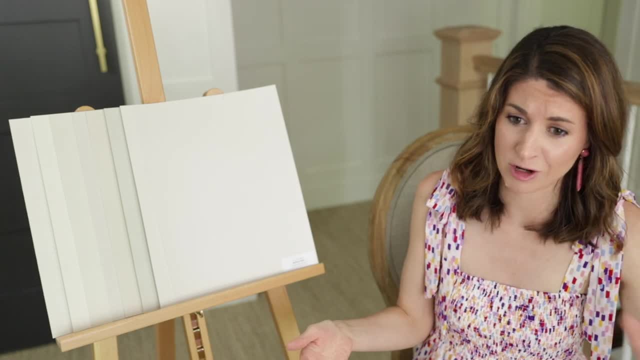 It's old or whatever, But the stone fireplace is definitely something that you need to look at. You don't want it staying and you're not changing it. You need to kind of look at the stone fireplace and let that dictate and drive your color decisions. 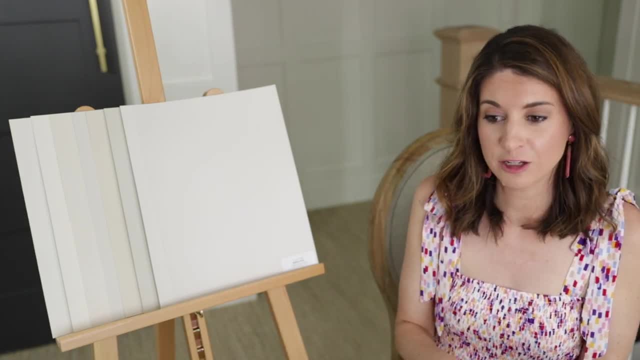 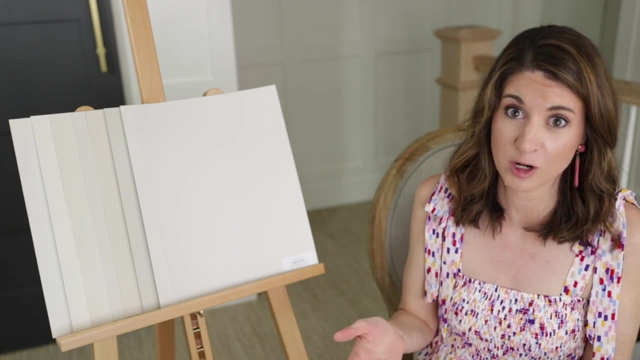 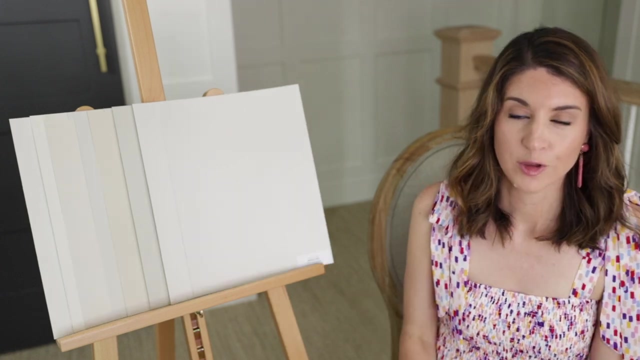 So just to recap again, look at your fixed elements, look at your furnishings, see which paint color, which undertone, best relates to those elements. And it's going to be a lot of trial and error and a lot of testing, But really that is the only way to make sure that you're happy with your paint color at the end of the day. 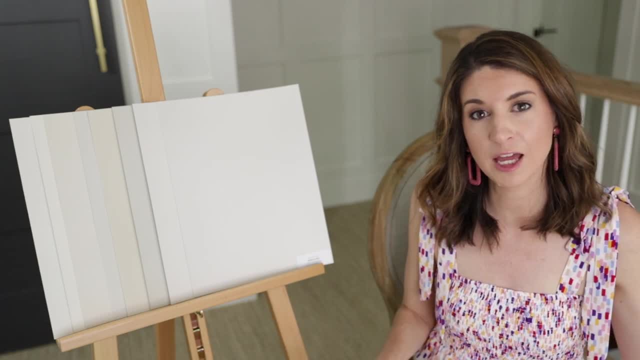 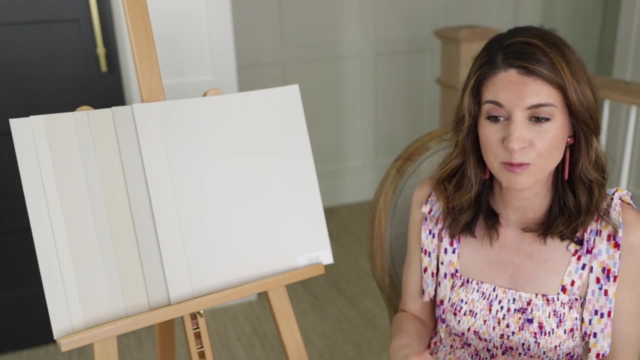 Okay, the next tip I have for you is to forget about those online inspiration photos. Stop going on Pinterest or Instagram and looking for inspiration photos of the color that you think you want, Because I can promise you that's always going to steer you in the wrong direction. 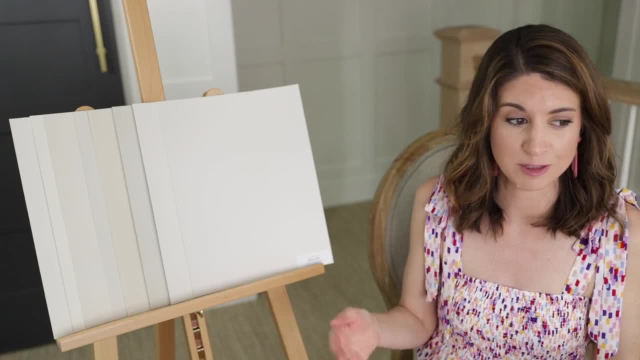 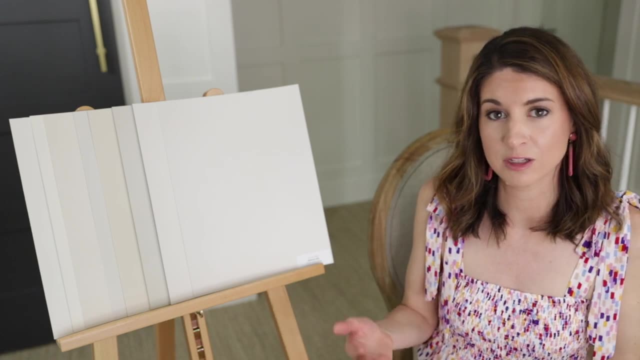 So pretty much every color that you will see online has been highly edited. The lighting has been affected. The lighting in the room- the natural light- is mostly going to be different than the natural light in your room, So you need to take those online photos with a grain of salt. 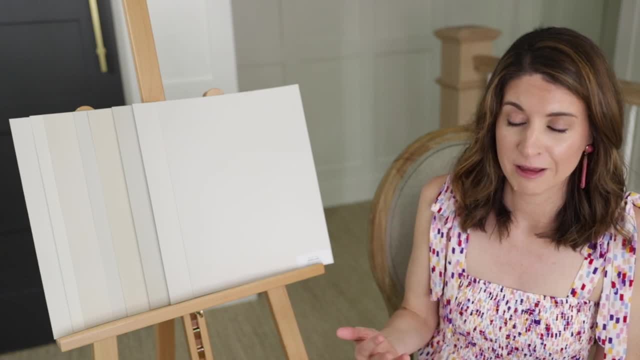 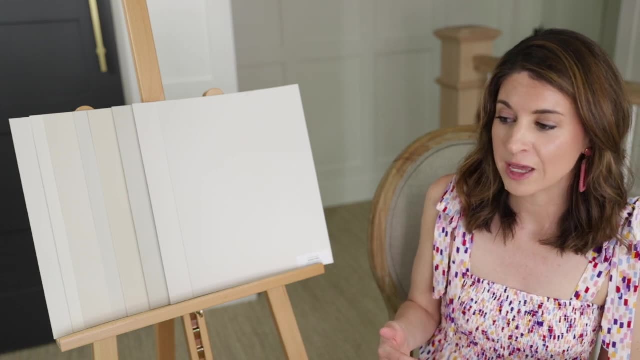 I know it's hard to do because people feel like they have to start somewhere. Just take those with a grain of salt and know that the lighting is most likely not going to be replicated the same way in your house. So that's why it's so important to test out colors in your home and see how they react to your lighting. 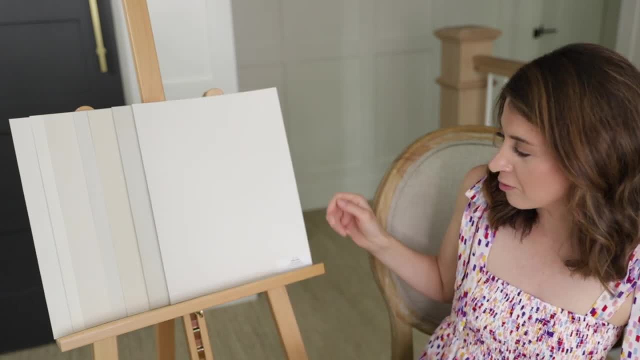 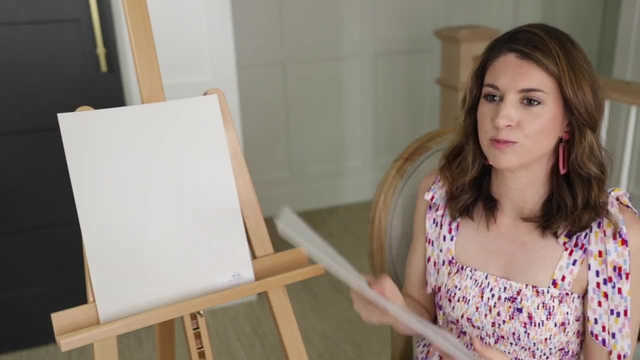 What you want to do is, when you have your paint colors narrowed down, do not- especially with neutrals, do not ever- just put them right up against the wall on your current wall color. That is going to skew your decision all day long. 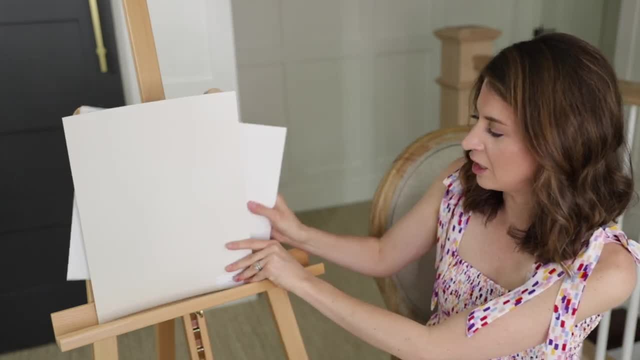 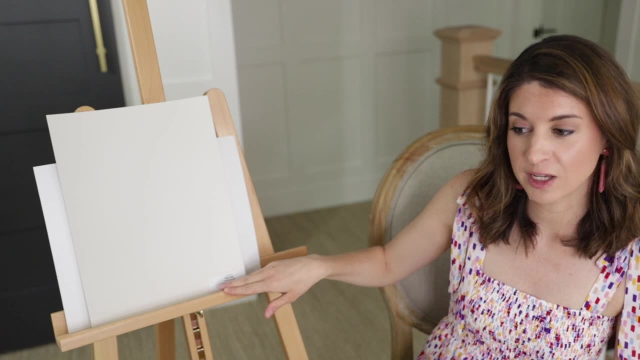 So what you want to do is you want to put them behind a sheet of pure white poster board, or you can use computer paper. These are my professional color samples, but you can kind of get that same effect when you use those peel and stick samples, which I have a lot of those and I love those. 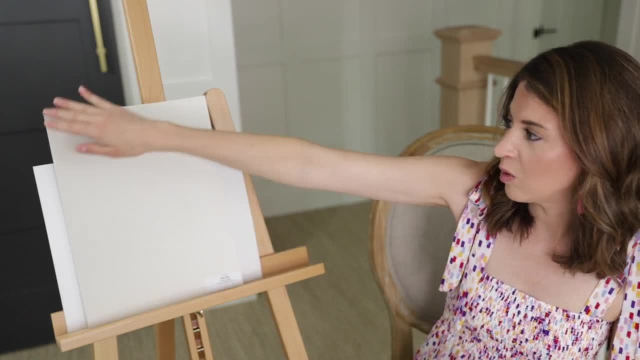 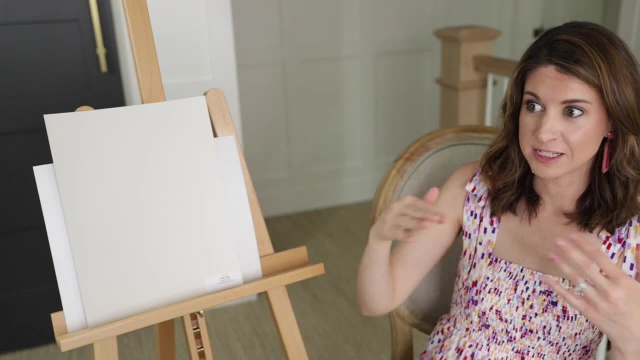 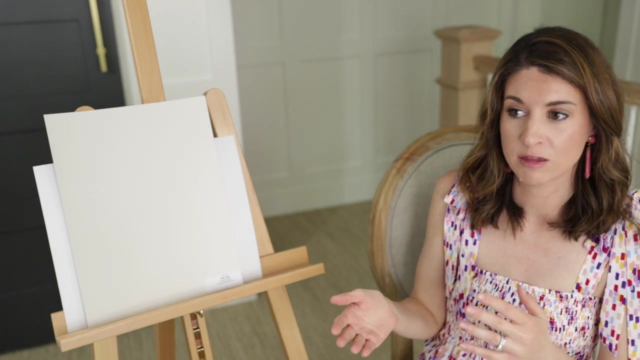 Put it up on a white poster board. Ideally you want a one inch border around the entire paint sample and then put that to the wall And then stand back and see how it reacts in your light. A lot of these colors say you've got a darker room with just one window and it faces opposite the sun.